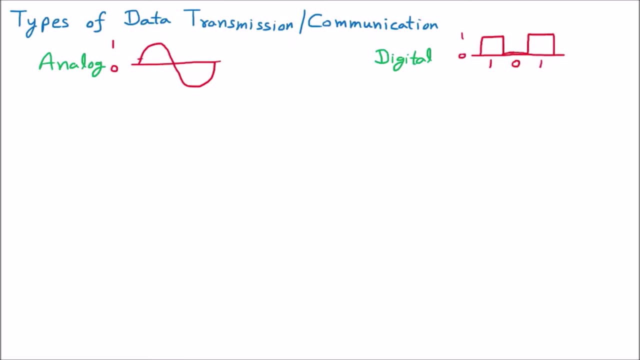 For example. then here there is another that is zero point one, zero point two, and so on. Multiple are there till one. Okay, Zero point nine. So multiple values are there between zero and one And there is only the zero and one values. So these are the difference between analog and digital. So we can easily conclude that analog signals can have. 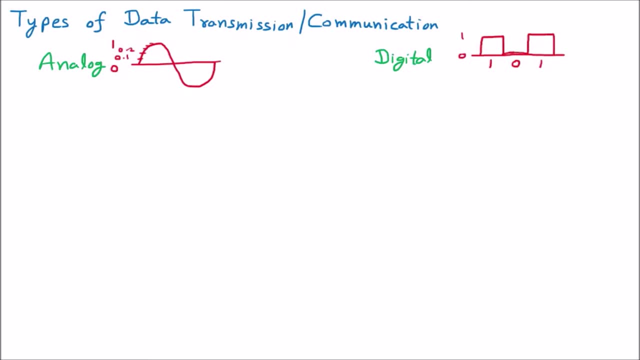 the values in the floating point. But the digital cannot have it only have the zero and one values. So we can say the analog signals are into the waveform. We represent the wave many times. So they are into the waveform in the form of wave. But talking about the digital signal, they are the on and off electric state. On and off electric state. 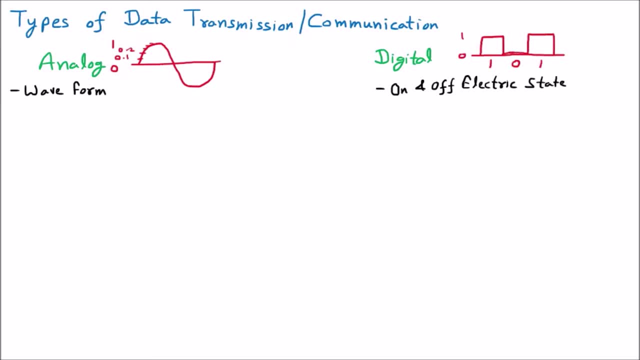 means they represent one for the on and represent zero for the off. Whenever we are talking about any digital circuit over there we are having on and off means you are switching on the fan or switching off the fan or switching on the IC, switching off the IC. So for that there is a signal: one for the on and zero for the off. We know that the 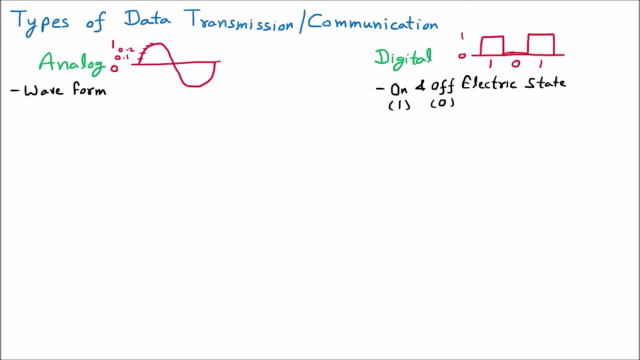 they are not stopping anywhere, Just like the analog signals are not stopping. So we can say that these are the continuous signal. Continuous means they are moving towards the end, But here we are having the full transition. That's why they are the discrete Digital, are the discrete signal, And some people also say that these are the distinct, Distinct means. these are the 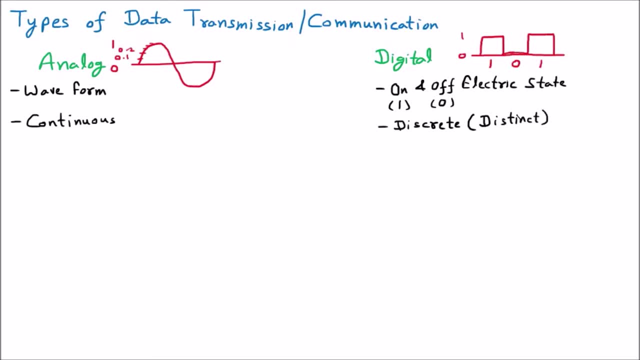 values, Two different values, Just like if I say between zero and one. there is a simple transition, Either zero or one in the digital, But in the analog there is a continuous transition: Zero point one, two, three, zero point four, zero point five, and so on. So that is very slow, slow transition. But here is a direct transition. That's why discrete, And they are represented by sine wave. 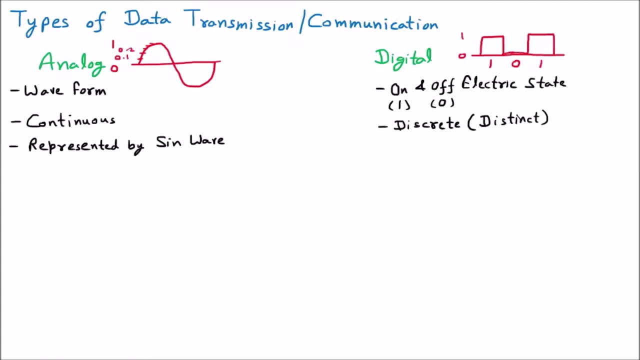 So the signal looks like the sine wave, Just like if we have gone through the mathematics subject. There are many waves which are present, which we use sine and cos Right. So sine wave looks like this. It is also the part of physics. Now, talking about the digital signal, There is no simple way to represent value like zero point two five, If you want to represent zero point two five. 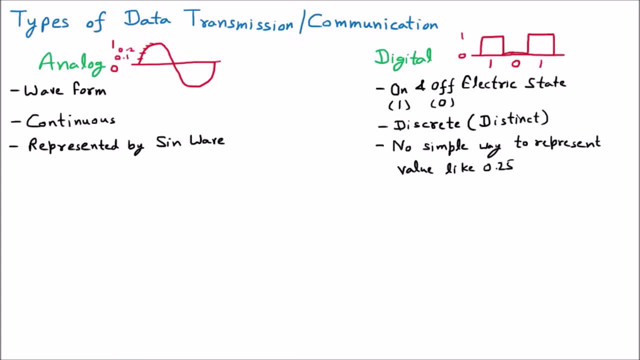 there is no option: either you will make it to zero or the one so point. floating point values are not the part of digital signal. well, the good thing about the analog is that analog device, analog device, means the devices which are using the analog. so analog device, monitor. monitor means they are going to measure. 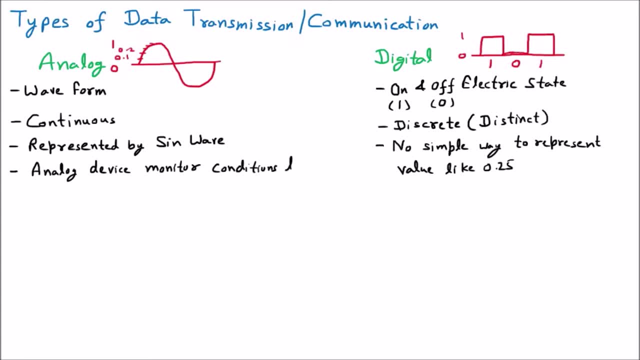 some conditions, like means they are going to monitor the conditions, like moment. moment means how we are going to move. something means what is the moment? example: if I am running right, what is my continuous movement? temperature, say. example, the temperature we are having in the digital form. we are having the. 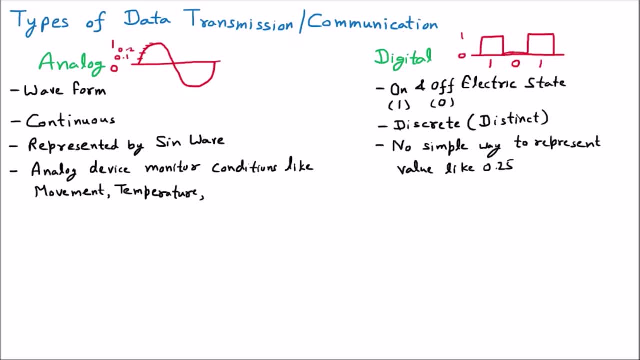 temperature like 13 degree, 14 degree, but in between there are multiple temperatures: 13.1, 13.2, 13.3, 4, 5. so all these temperature are measured in the analog form. so temperature is the quality of the analog, just like in a thermometer we. 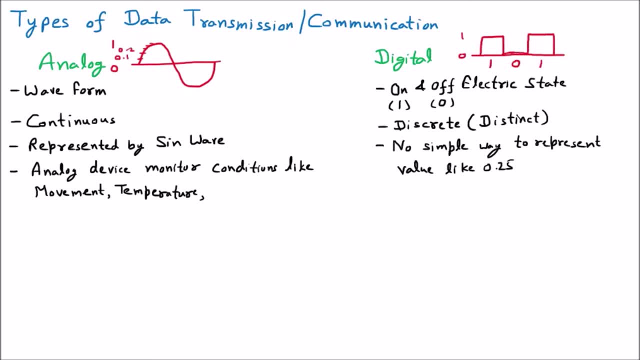 are having the temperature many times: 98.7, 98.8, right? so this is the analog signals we know, but here we are representing in the form of some digits. that is a different issue, because today we are having digital thermometer, but I am talking about the analog thermometer. 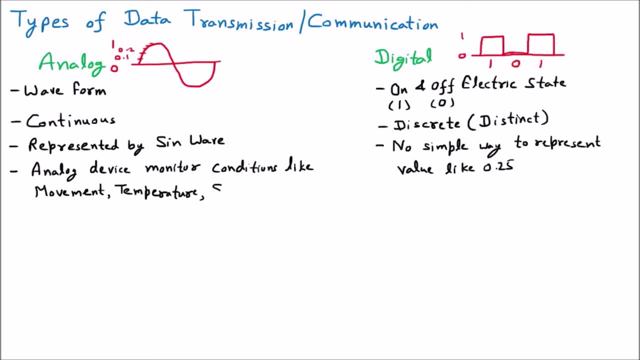 about this, okay, tomorrow, so that Al we are coming after 12 higher volume at 60 usu and tiers about the tone sound. spicy Jadi, EU音録音的不在mercode1广ro. 10. sound always can be invariant, likes like from slow sound, medium, high, high sound is always going to be in variants, likes like slow sound, medium, high, high sound is there, so this is the analog signal. but if I talk about it在低 attracts低, 5, low and one, so the sound is given an analog signal. so if I talk about the digital, now in theesta digital, there is one additional. 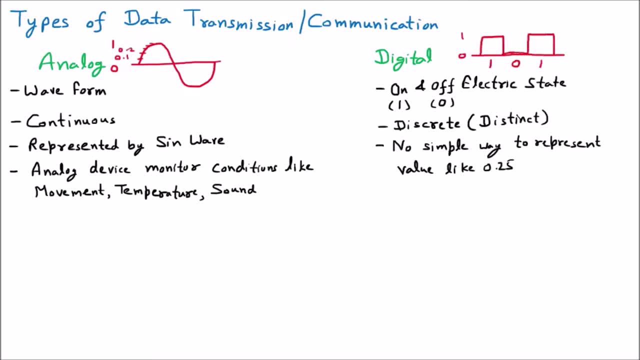 digital της数NO, digital in digital. there is one additional, which is very important: we are going to convert all the things to the digital form. let us suppose that the music information voice, because we know that music and voice are the analog. so how to take this side? digital, so music voice. 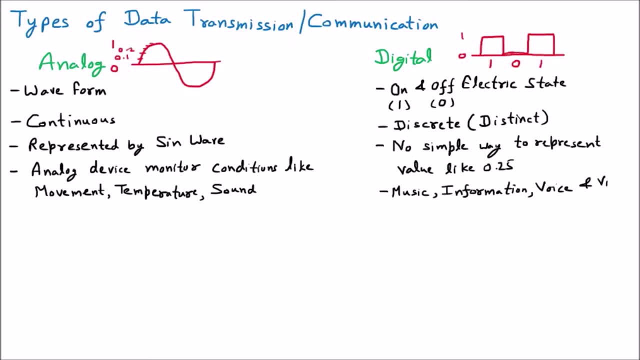 and video. video also contain audio, so video converted to binary binary means zero and one, so binary digital form can be Electronically manipulated. now the meaning is that whenever we are converting some of the analog signals, like music, information, voice video- because these are the lock- Oh to the binary digital. binary digital means zero and one digital form that we can manipulate them. 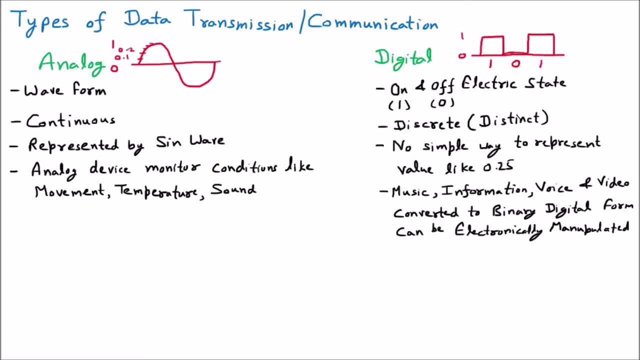 electronically. with the help of electronic devices, we can change them and also we can preserve preserved means. we can save them and regenerate. it means one they are converting to digital form. it is very easy for us to electronically make the manipulation. preserve them means save them somewhere or again generate them. so that is the main quality of the digital, so what we have. 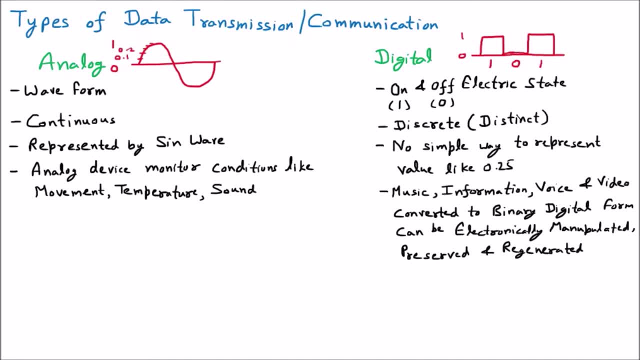 learned from the analog and digital. the thing is that analog is the waveform in the continuous waves or the sine wave and temperature, pressure, sound, movement. these are the analog signals. digital r 0 and 1, discrete, but there we don't have the 0.25 any. any representation is not there, like 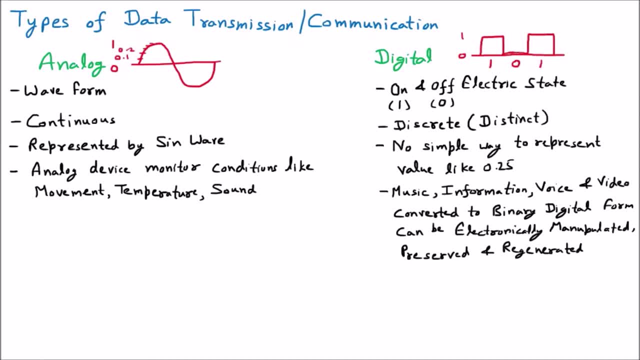 but once we are converting analog to digital form then it is very easy for us to electronically work with them. now we are going to take some examples of the analog signal. so if we talk about the example in the first example which we are having is the speech. speech means if i am talking to 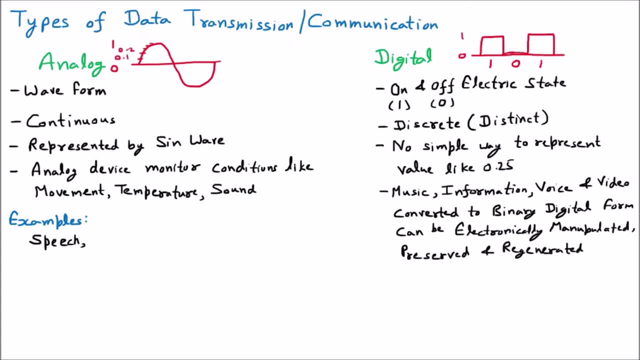 you in the continuous manner. that is speech. it is analog signal voice on telephone. on telephone we use to talk with each other, right. that is again the example of analog or even the analog watch. many times we are having the watch on the wall clock which is unlock. 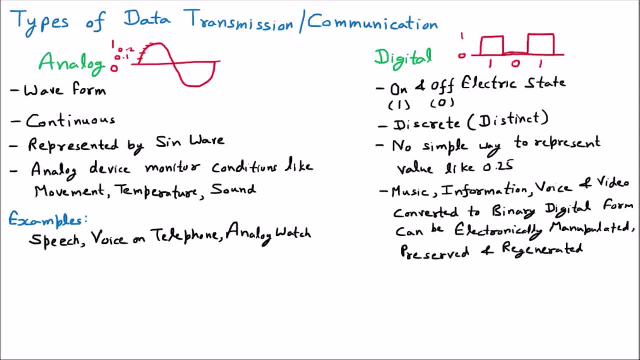 where the dice is moving right. it is not like digital watch. so that dice is moving right and this is becoming between 12 then 12.1. two, three, four, then becomes one. one point. two, three, four, three, four, then two. right, so this way it is moving. so that is a analog watch, or now we're taking the 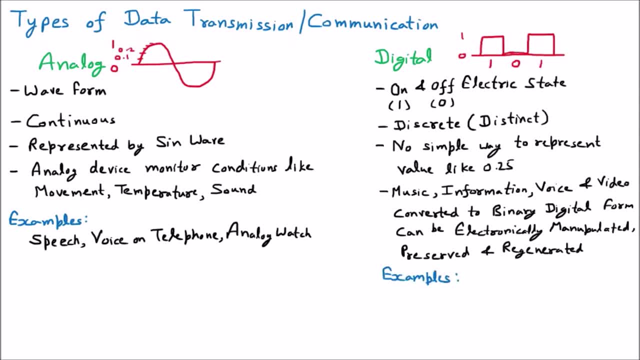 example of the digital. so the example of digital is digital watch. we know that today is the trend of digital watch and we are having the accurate results right there. we are having the direct conversion. there is no the floating values in between. there is a direct value coming. 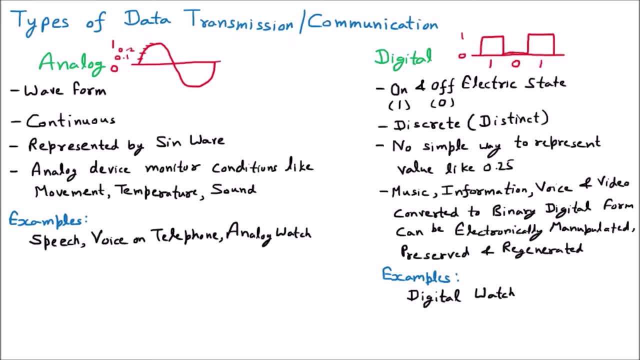 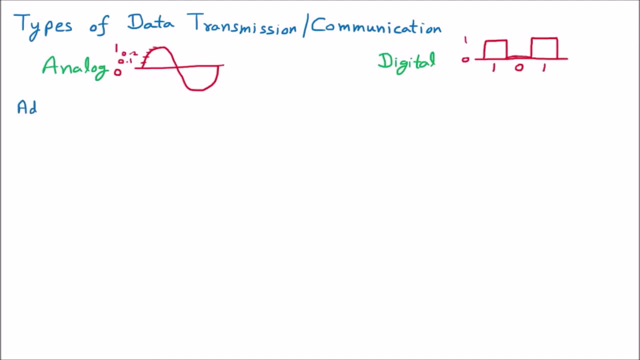 right, there is no digits or point value. so that is a digital watch which we are having now. we are going towards the advantages of the analog signal. so now we are learning the advantages of analog communication. if i talk about the very first advantage, or if i say it: 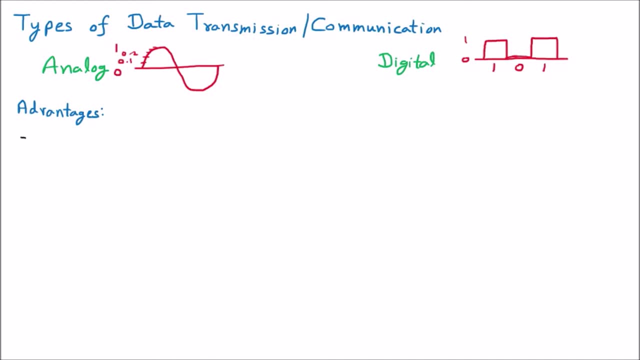 is the normal one advantage of the analog signal, and that is that it is having the capability to capture the subtle nature. subtle nature meaning something is continuous, if anything is moving constantly, so that nature is called the subtle nature. so subtle means which is going to continuously vary. 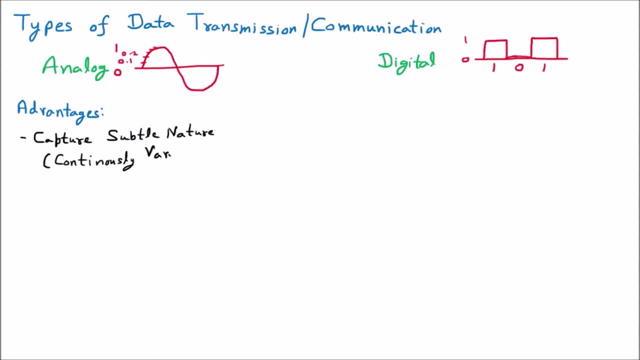 so if anything is continuously vary, like our temperature, pressure, sound, that can be measured very easily with the help of the analog signal. that is the only advantage of analog signal. now, if i talk about the disadvantage of analog signal, so disadvantages. the first disadvantage of the analog signal is that they lose the energy after certain distance, means, if you 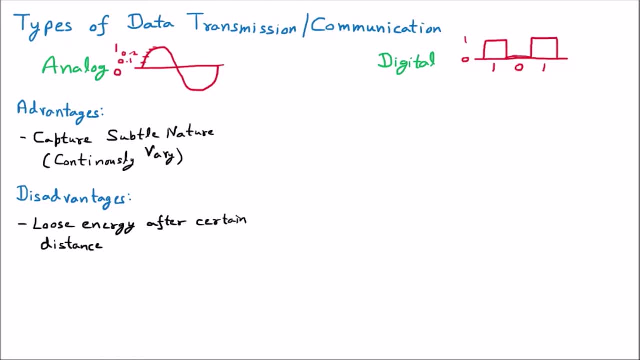 are sending the analog signal from one station to another station, then after some time, at some distance, it will lose the energy, and we know that in the networking we are having a device that is repeater, that is used to amplify the energy. so there we require the repeater. one more disadvantage of the 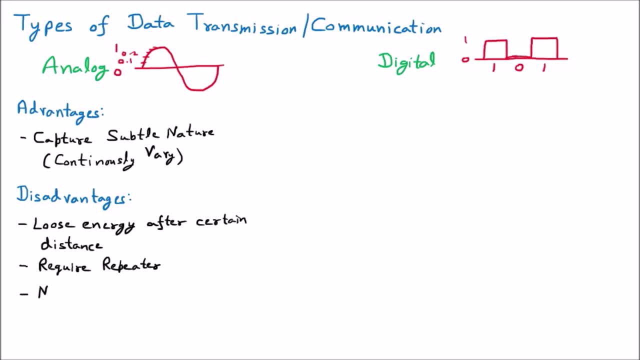 analog signal is that they are having the noise, so they are noise prone means they can capture the noise very easily. if they are moving from one location to another, then if some noise is in the between, so noise is merged with the analog signal. so that is a problem and very disadvantage of the 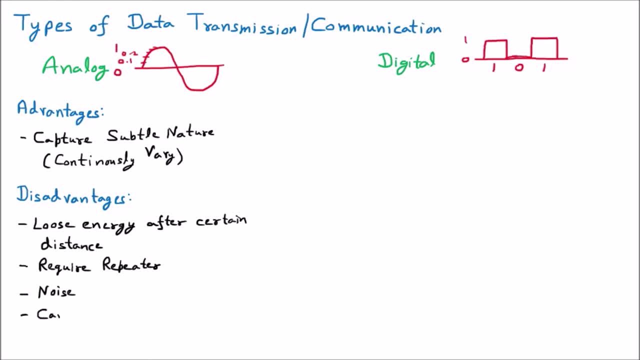 analog signal which we are having is the. it can't be copied perfectly. let us suppose that you are having some kind of data in the analog signal and if you want to copy, not possible. if you are assuming that there is some kind of movie in the analog form, you cannot copy them perfectly. 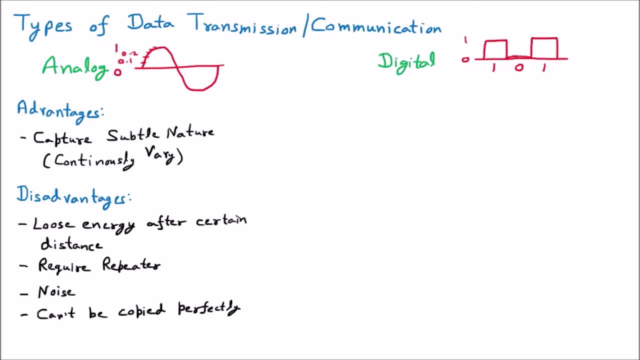 there will be the distortion 100, so that's why for the copy purpose we cannot use analogs. example: i am speaking what, what it is there? if, then, if i am copying directly, the same voice will not coming at your system. so what is going on? because i am speaking and you are understanding still my voice. 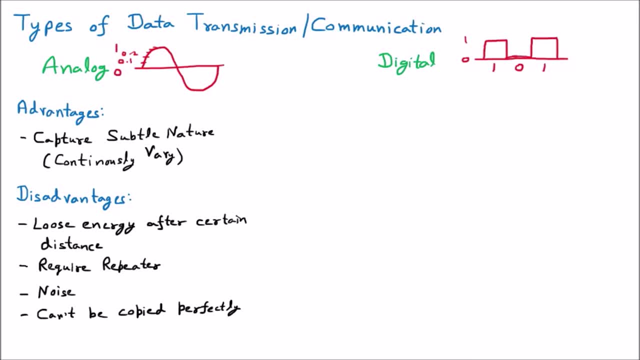 is the analog and you are understanding the same voice, because my voice is first converted to digital, then it is sending to you, then again the speakers are coming back to the analog. so that is the communication going on. the communication through the network is the digital because if 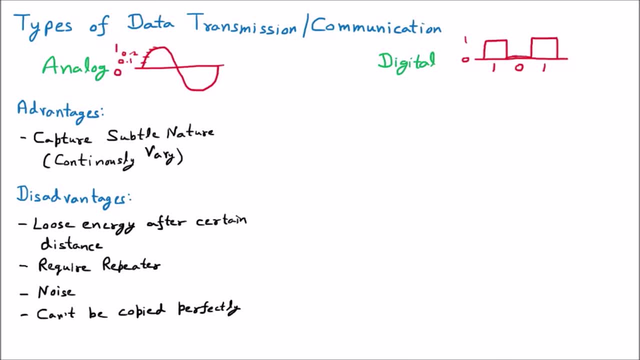 i send the analog signals directly. if i'm sending my voice directly, it will not reach you because the intensity which i am talking, or the amplification, everything will be digital distorted. so that is the problem. so that's why we can say that there is distortion in audio and video. today these things are very, very much popular. even we are using the whatsapp. 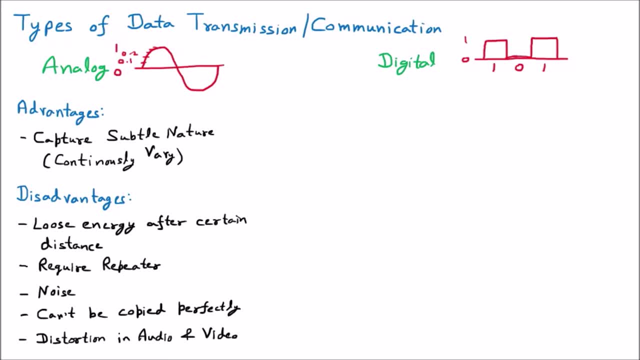 facebook, anything. audio and the video. these are main popular because video is also the combination of various frames, right? if a video is moving, there are various frames behind the video. so that is why we can say that there is distortion in audio and video and that which are running. right. so this is again the analog and my voice is again analog. so these 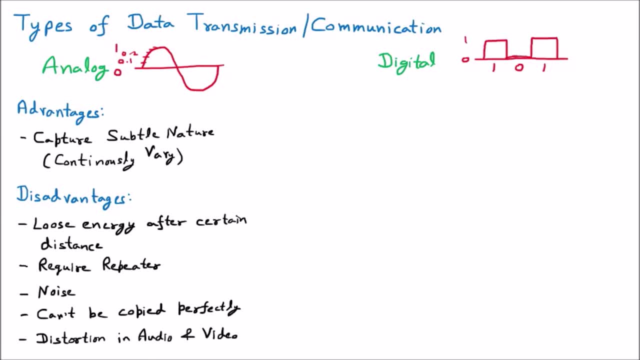 will be distorted. so now coming to the advantages of the digital communication. so, talking about the advantages of digital, there are various advantages of the digital communication. the first thing which we are having is the fast communication. if i compare with the analog signal, then the digital is very fast. sending the data is very 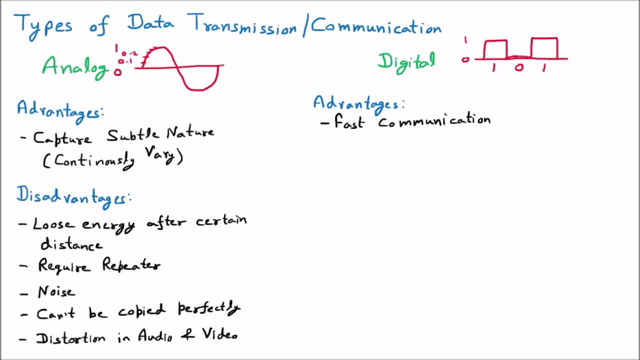 fast. you you know by yourself, because there are two things, zero and one, and in the analog there are many things: zero point one, two, zero point three, zero point four, and so on. so sending zero and one is very fast, so it is a fast communication. then afterward there is perfect copy means, if you 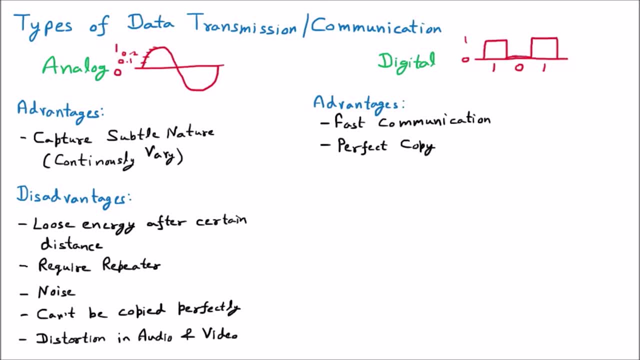 are going to copy the digital signal. there is perfect copy and it is not only the three, two times or hundred times copy. no millionth copy is having the same as original. let us suppose that you are having a movie you have given to your friend, friend given to another friend again. 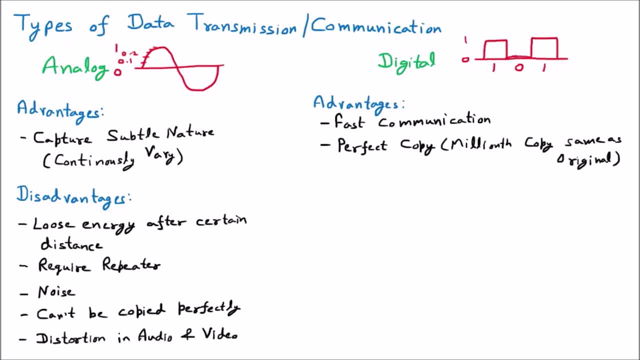 another, another, another million times movie is given, same will be there as it was the first. so that's why the digital is very much popular. also, it is very high speed. so for the high speed communication we use the digital signal and also it is of high quality, just like the audio you have. 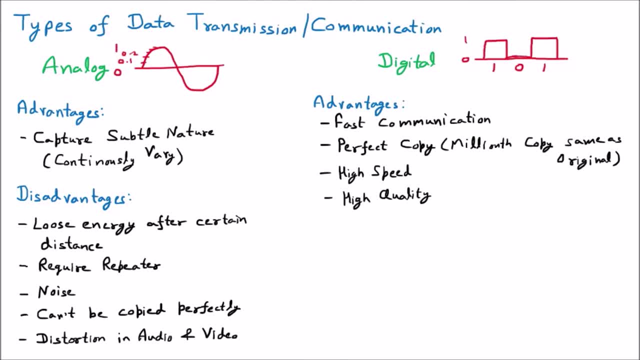 seen that many times. the icon is there: dolby digital- because the dolby is giving the sound of digital quality, high quality. so this is how the digital communication is going to be. so this is how the digital signals are there and they are giving you the complete 1080. even today, we are. 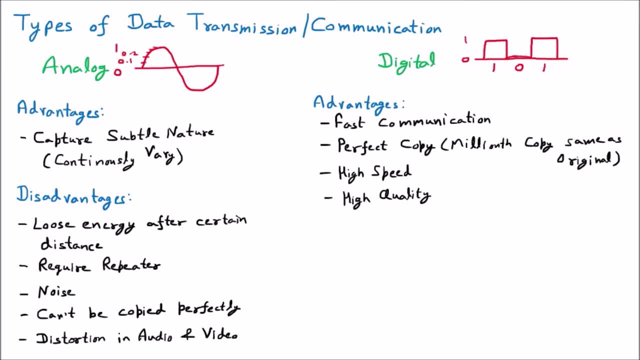 having the ultra definition pixels right. so oled tv, so what they are, they are working on the digital form. that's why they are giving you that much quality right. so that is the digital communication. more advantages of digital are there. they are less prone to error. well, it is obviously to understand if i am sending a zero and one, two things i am sending. 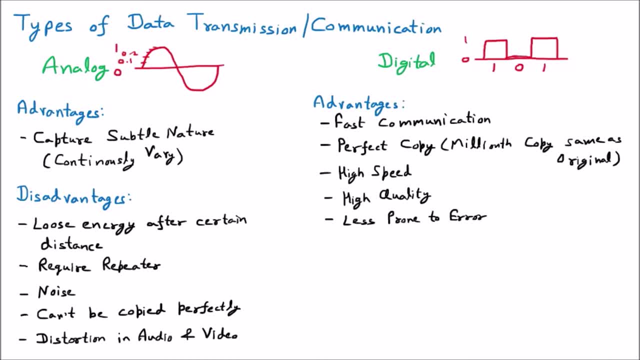 less error will come. but if i am sending many things- zero point one, two, three, zero point four, five, six, so on, so that is for sure the error right. so digital is having the less prone to error. again, they are very much accurate and reliable. we can rely on the digital but we cannot rely on the 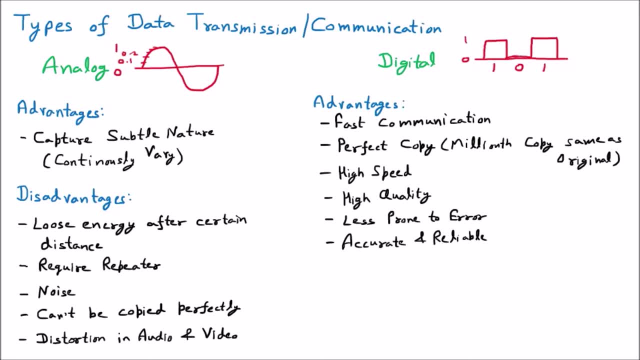 so these are the various advantages of the digital communication. now talking about the disadvantages, so disadvantages of digital communication. the first disadvantage, or we can say the only disadvantage of digital communication, is that they use absorber and regenerator. absorbers and the regenerator means something we are understanding, is something is going to absorb the digital signal and 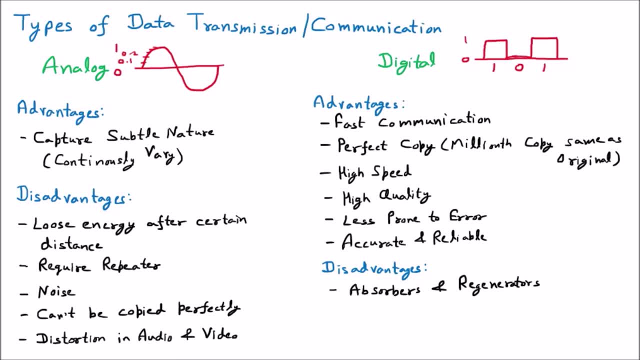 regenerate them. why? why not use the repeater? because repeater amplify the signal and in the digital there is only zero and one. what we can amplify, we cannot make one as two. no, so digital signals can't be amplified. so first of all, we must know that digital signals can't be amplified. 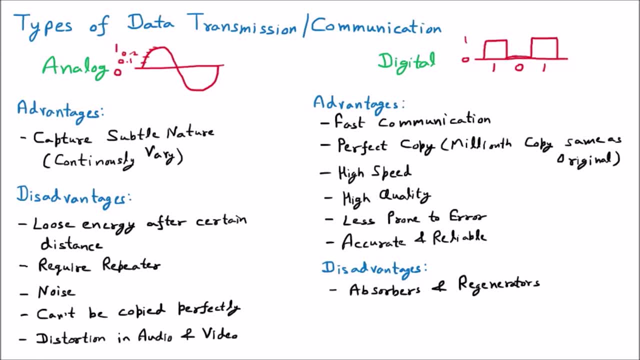 and one more thing: if i am sending the signals at the long distance, obviously signals get distorted slightly. so first thing we are learning is that digital signals send at the long distance distorted slightly, and for that we don't use the repeater because we cannot amplify one to two. so there we. 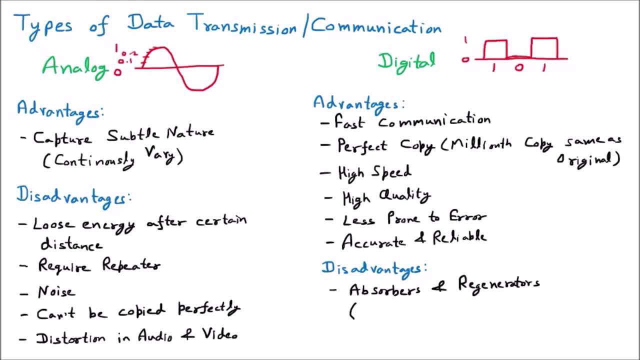 use something, device which is going to absorb the complete signal and regenerate them at the same. so especially if those ingredients will be destroyed or used. when we talk about digital signals, then only the cieot circumstances, that continously they are required, and this is because이라고. 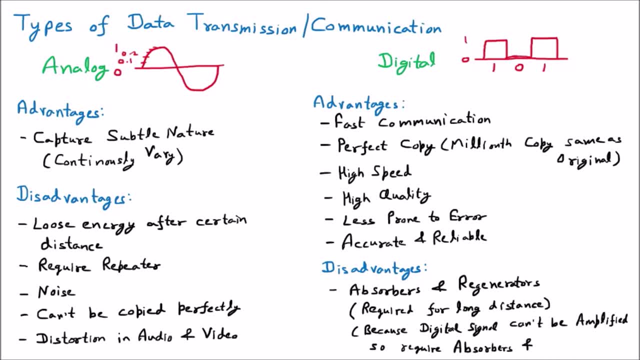 completely absorbers and regenerate them completely. so that is the thing that is the only disadvantage of the digital communication. so what we have gone through in the advantages and disadvantages of analog advantages is that it is going to capture the subtle nature means continuous things we can easily capture. disadvantage is that after some distance, 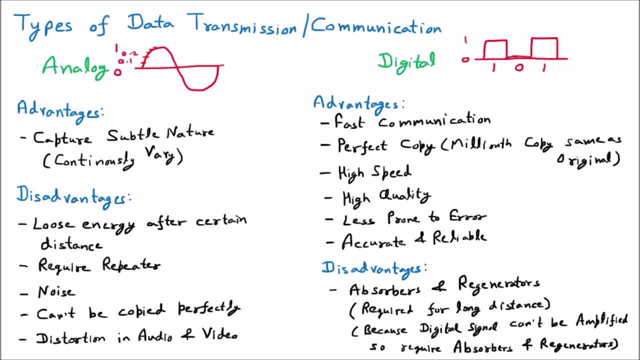 it's lose the energy. it require a repeater. they become the noise. then we cannot copy them. distortion also come in audio and video. so the solution is the digital signal, in which we are having advantages like fast communication, high speed, high quality, less prone to error, accurate and reliable. so all these things are there. even we are copying millions. 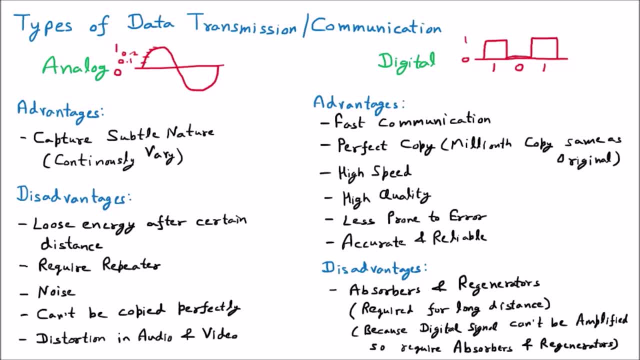 of the times, the copy is same. so all the movies which you are having at your home or which is on your Tata Sky or maybe any other device, they all are into the digital form. otherwise the quality will not be the high definition or full HD which we are having right, and the disadvantages are they. 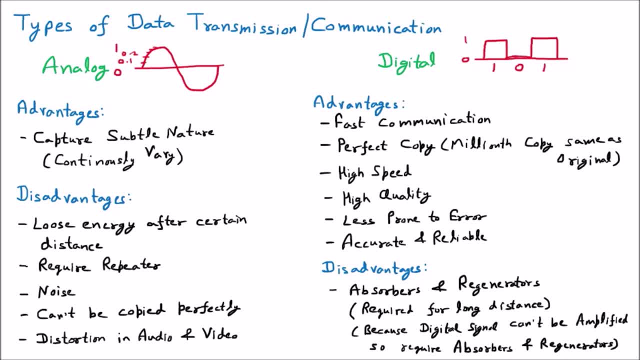 need the absorber and the regenerator. so that is all about the types of data transmission and communication you.